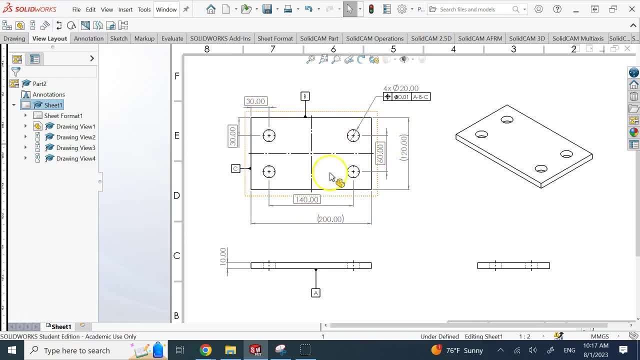 need to go into all of these dimensions because this part is simple. but if the part is bigger and it has so many features and the machine is had to stop and add and subtract a bunch of things to finally he finds the total size of the part, that is going to take some of his time or her time. 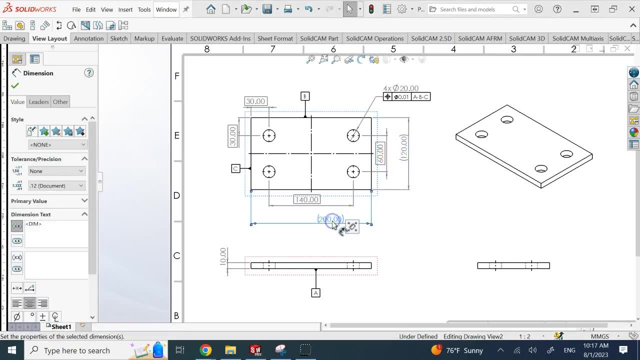 so he has to add and subtract a bunch of things to finally he finds the total size of the part. that is going to take some of his time or her time. so he here for convenience. i add them here, but by putting those parentheses around it i'm telling. 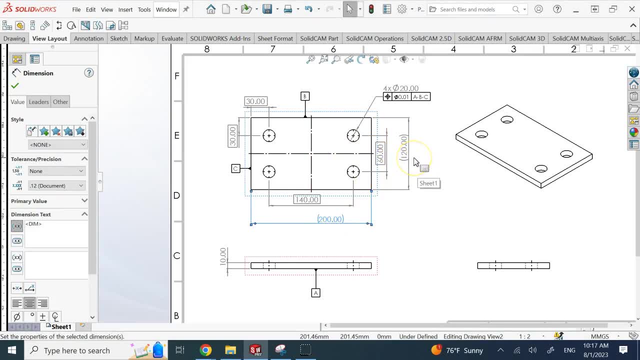 them that, hey, you can get this from somewhere else, but i'm just putting there for you. so, although it's redundant, it's okay to have them now. in order to make a dimension reference dimension and add parentheses, all you need is to click on that dimension in solidworks. 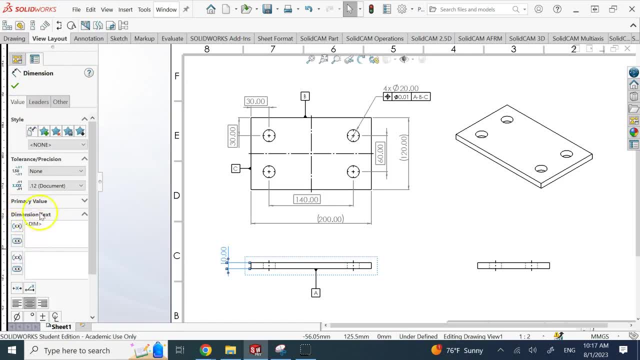 and then here you see this option on this dimension window, next to the dimension text. it says what it says: add parentheses. so if i click there, you see i have added parentheses and i can also what turn it off. so this is how you make a dimension. what a reference. 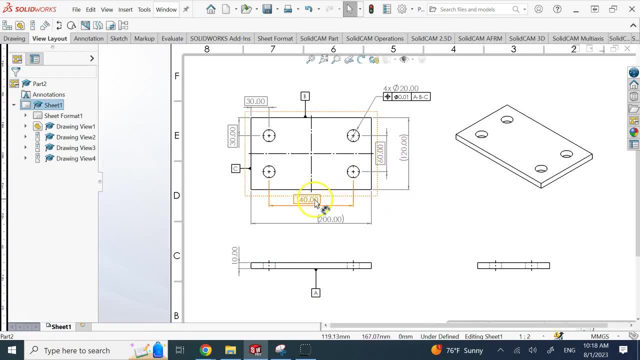 dimension. the next type of dimension you have are the ones inside these rectangular boxes, which we call basic dimension, and basic dimension is a dimension that is typically used with a true position- uh, gdnt or feature control, frame right, fcf- and it is going to provide the true theoretical 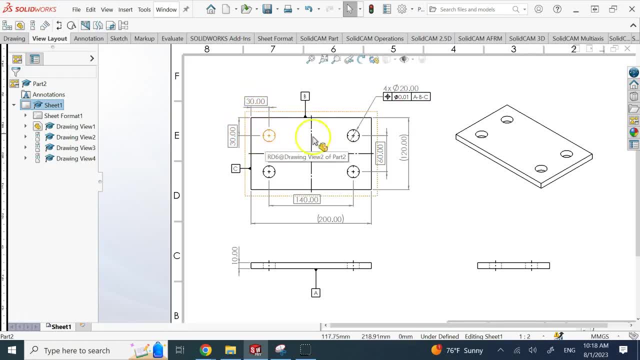 position of a feature. so here let's say, i want to know the true position of the centers of these four holes. so how do i find it? well, i ideally want the center of this hole to be drilled at 30 and 30 with respect to this corner. okay, by fixing uh surfaces a, b and c, the bottom, back and the left. 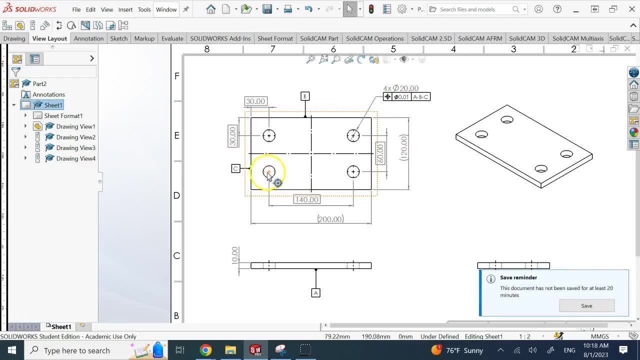 surface onto the inspection table, and then these other centers can also be found. using what? using a? okay, so using these four dimensions, i can theoretically find what the intended locations. okay, if i write an object in here, i could not find all of these. L Firma two黑. here is a or I know, look, erre, and I'm confused. it would take time to find all these lo and they and i'll write 3 and if I figure they're not enough, maybe 5. Україl, from here i'll go thick you. can't even hit that H was 형 the point, I just ignore it in a minute. um the point here. thisückt this people just advice here and that it its not real thing. otherwise it was a really simple look up if next to this point detto xaq and that todaul. here is the position that i got. so 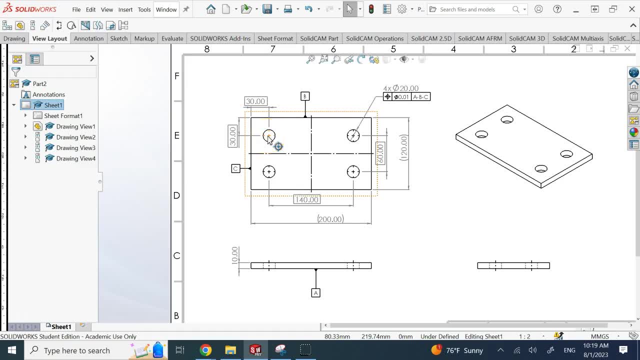 letsる operation data. okay, that x is seperti 레� settlement. i can tell them work what by anniversary for the centers of these cylindrical holes. okay, now how much am i allowed to deviate when i drill the centers from these theoretical centers i provided using this feature control frame and 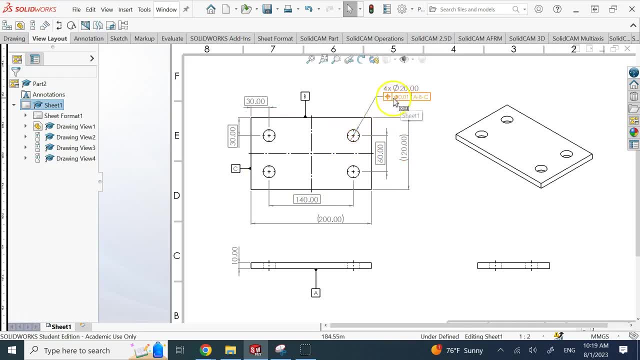 i say hey, first of all, those are cylindrical holes. you see, there is this symbol diameter here and the amount, the radial distance that i'm allowed to deviate, is only 0.1 of an inch. okay, so 0.01 off radially from these theoretical points is how much i can be off when i use my. 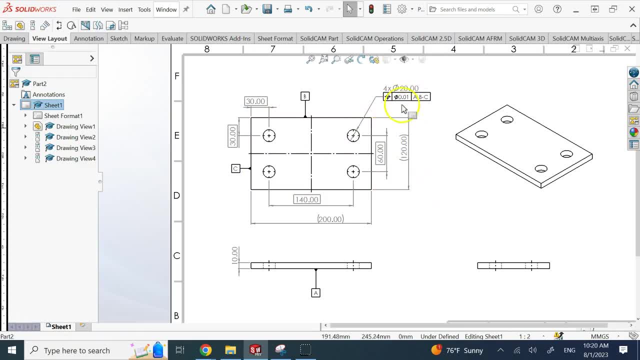 datum features a, b and c: okay, so the amount of deviation is reflected here, and so for these four dimensions i do not need to provide what any tolerance. if i have a dimension like this, the tolerance for that, that is not a basic one, the tolerance for that should. 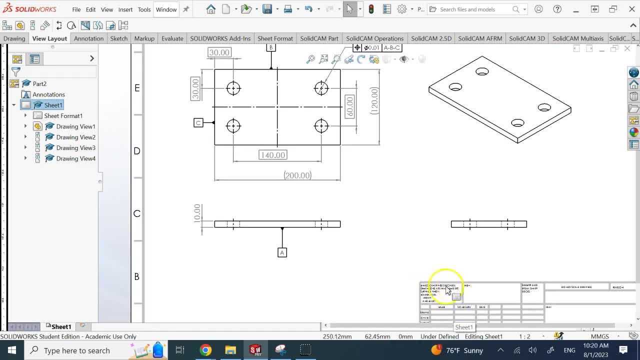 either be provided here in the general tolerance node in the design table, or if it doesn't follow that tolerance, then i have to come here and what i have to manually add it so say it's a bilateral one and it's like plus one and minus, plus 0.01 and minus 0.02. okay, so i have to either provide that. 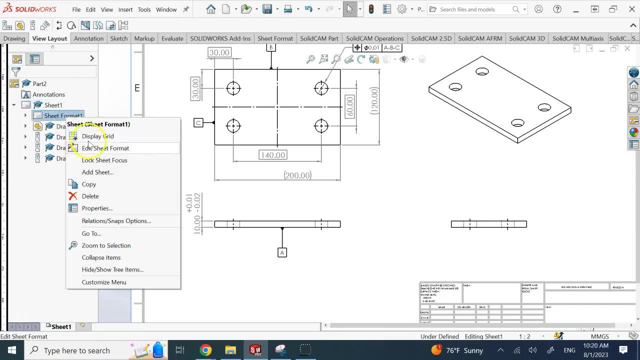 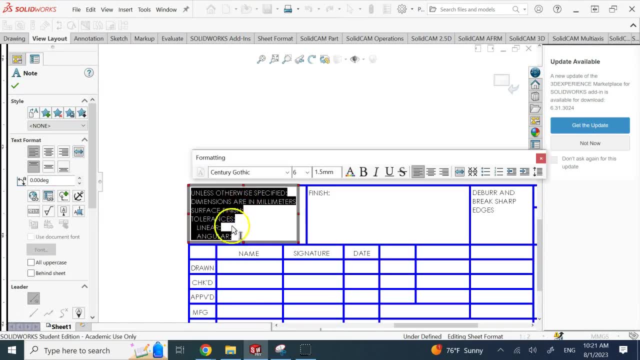 tolerance here. or, as i said, you can go right click here, go to edit sheet format and then go to this tolerance node and say what, unless otherwise specified, then for linear dimensions, then it's what plus and minus, uh, let's say uh, 0.01, okay, something like that. and then for angular degrees, 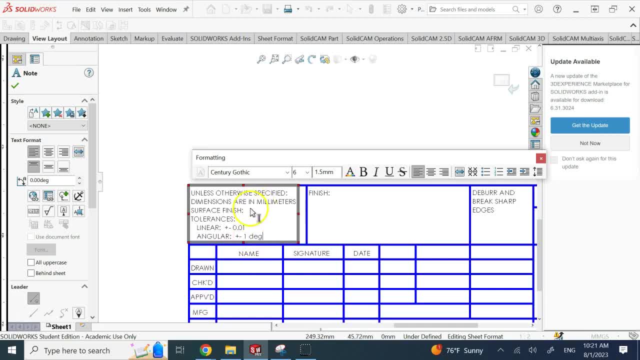 is like plus and minus one degrees, and then all dimensions are in inches, for example, or in millimeters or something. okay, so uh, this way, any tolerance other than the basic one, other than the basic ones and of course reference ones are just really there for uh convenience. so, other than those, any regular dimension has to follow plus and minus 0.01. 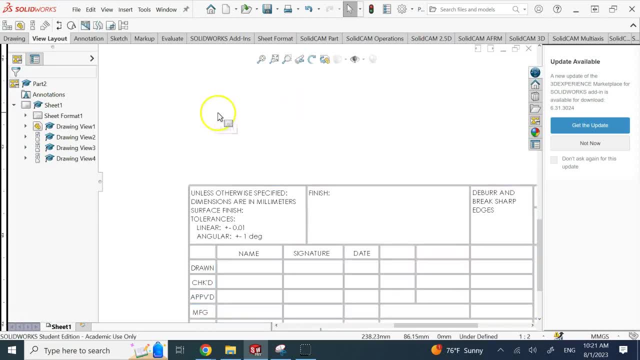 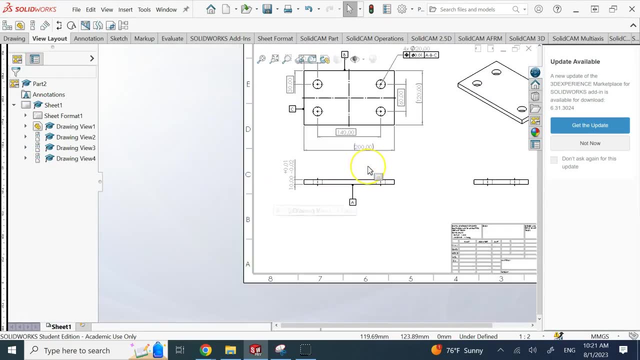 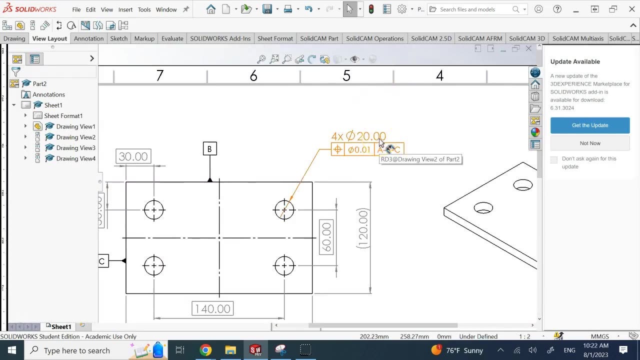 unless otherwise specified, like this one. this one is different, so for this one it's what it's, plus 0.01 minus 0.02. then that plus minus 0.01 is observed where here, for example, for this diameter of 20, it could be 20 plus and minus 0.01, and i don't need to basically provide it here. 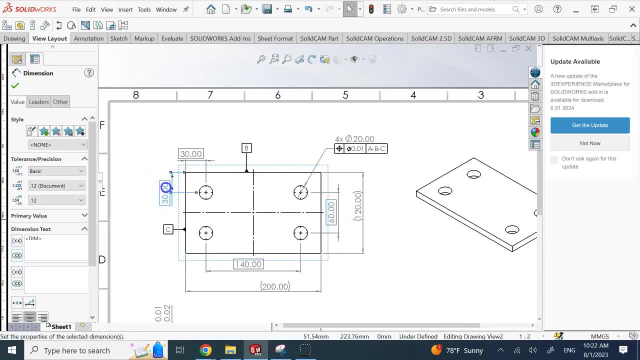 now, as i said, these basic dimensions don't have a tolerance. okay, because the tolerance for those is reflected here in this cfc. so, in order to make a dimension a basic dimension, what you need to do is, when you go to a dimension, let me. let me add it here one more time for you. so, 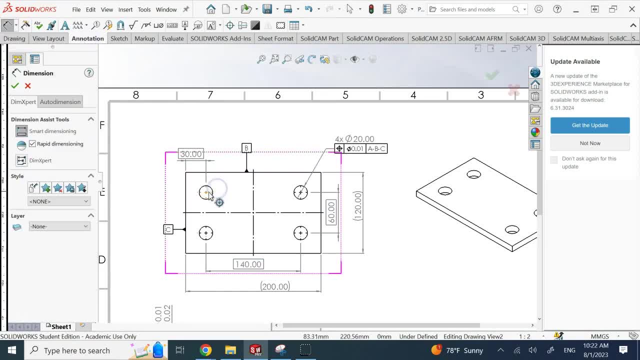 uh, you go here and add a dimension, right. so let's say you go here and here and add this dimension. then, instead of adding a tolerance for it, or say none, or say bilateral, you say what: i want it to be a basic dimension. and there we go. 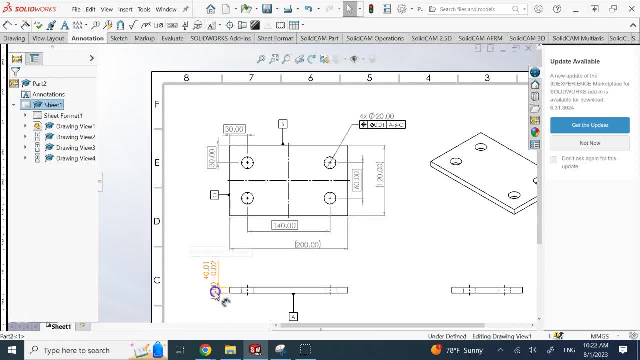 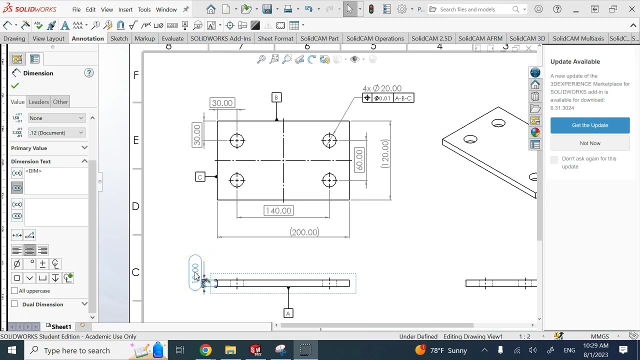 okay and it's different from, uh, this here. okay, uh, that you can put basically what you can do an inspection dimension. that is a separate thing. an inspection dimension would basically tell the part inspectors in a factory to how frequently inspect some dimensions for their tolerances to make sure their tolerances are met or not. okay, so they need to basically get statistics. 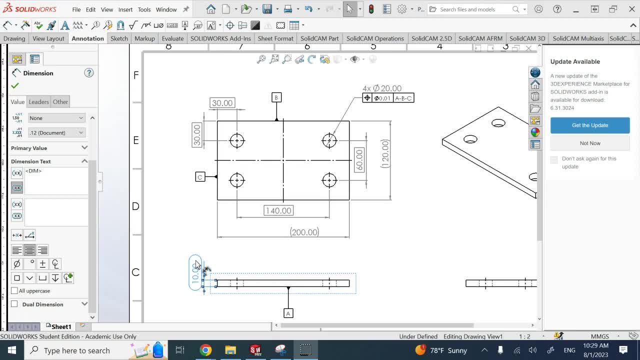 from those dimensions for quality control and so on. so, as i said, if you put something inside this uh, rounded hole- you might call it or slot- then that is different from a basic dimension, and one of the things that you can typically add to this dimension text is how frequently, as i said,